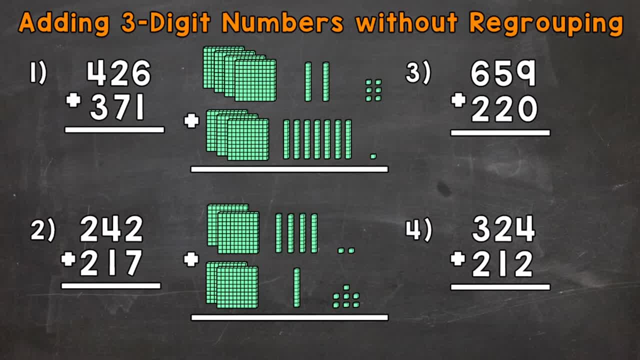 426 plus 371.. I have some base 10 blocks to the right of the problem to help us visualize exactly what's happening as we go through this addition problem. Now, when we add, we always start with the ones place, so 6 plus 1.. We can see that right here: 6 ones plus 1 one. That's going to. 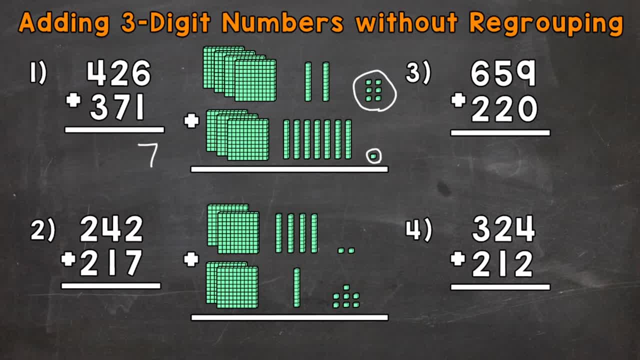 give us 7 ones, Then we have 2 plus 7 in the tens place. That 2 has a value of 20, and the 7 has a value of 70. Because the 2 represents 2 groups of 10 right here, so it has a value of 20.. And the 7 has a value of 70,. 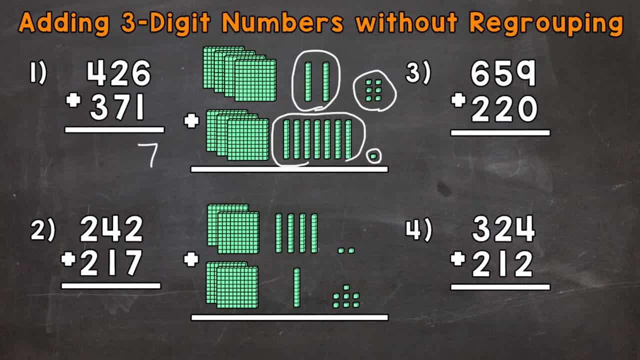 because it represents 7 groups of 10.. So although we're doing 2 plus 7 to get us 9, here, it's actually 20 plus 70, because those digits are in the tens place. Now we end with the hundreds place, so we 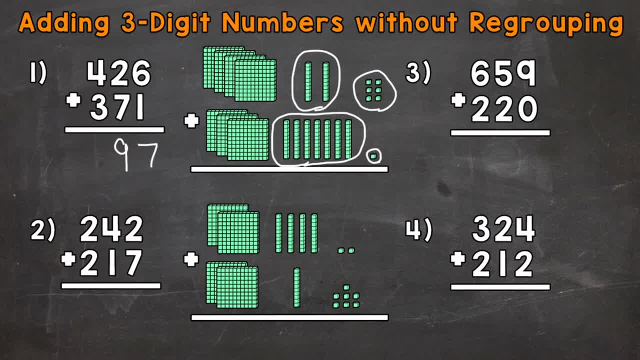 have 4 plus 3.. So 4 represents 4 groups of 100, so it has a value of 400, plus 3 groups of 100, which has a value of 300.. 4 plus 3, or 400 plus 300, gives us a 7 in the hundreds place. That 7 has a value of 700. So our 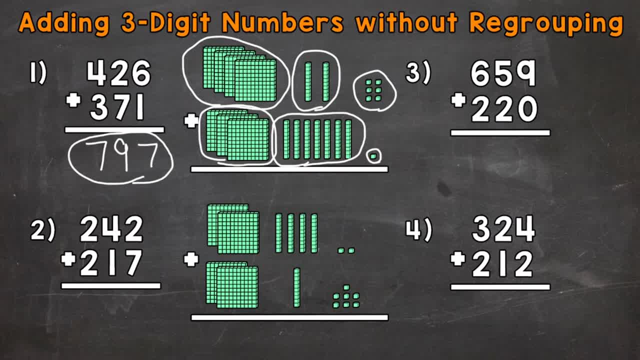 final answer is 797.. Let's move on to number 2, where we have 242.. Be ready with our currentization question. Our final answer is 3.. We came up with the twoいう times В draw earlier, So those Incredibilist areas have 0 or W. 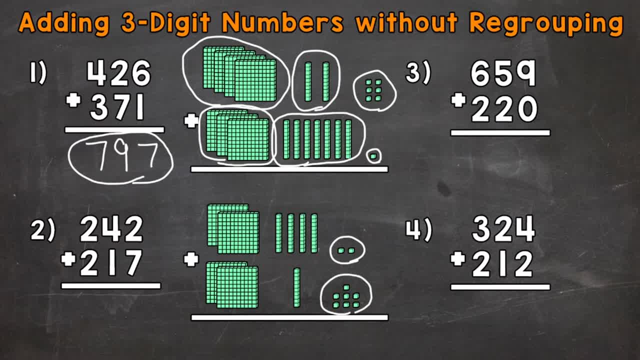 The specified areas, give us 2 plus지를. The same way that we'd draw here is that we'd take the tranquility figure and Aristoteles' one would give us 4.. So 4 groups of 50, or assuming the answer will be 0.. 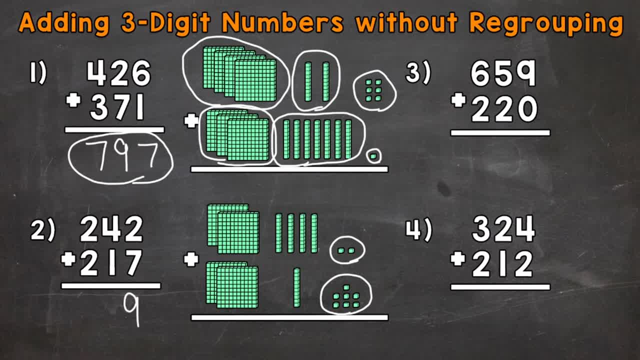 Then we add 2,, And so we have 342 pigments, which gives us 211.. So the rest of the 5 will be 7,, plus that and that and 6.. And of course we'll have 2 more minutes to do this question again. 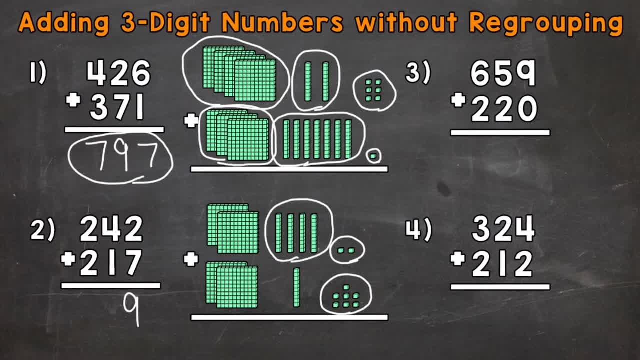 Remember, always start with the ones. So 2 ones plus 7 ones gives us a total of 9 ones. We have a 9 in the ones place. Then we have 4 plus 1, or 40 plus 10.. so that's going to give us a 5 in the tens place. 4 plus 1 is 5, or 40 plus 10 is 50. that 5 is in the 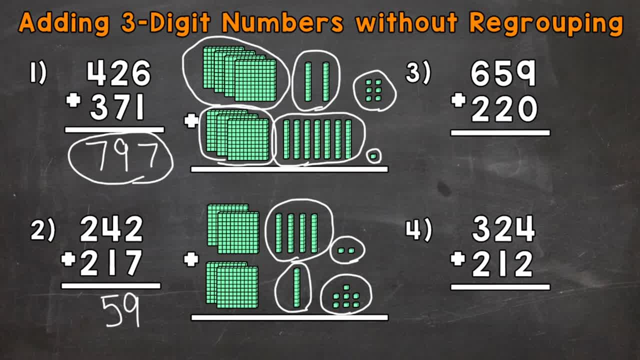 tens place, so it has a value of 50, and then, lastly, the hundreds place, so two groups of 100, which has a value of 200, plus another two groups of 100, which has a value of 200, so that 2 plus 2 gives. 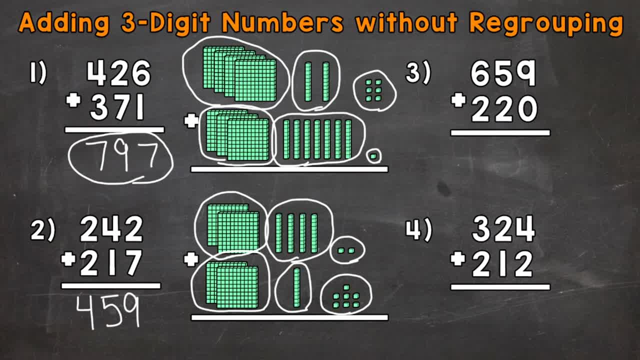 us a 4, which represents four groups of 100 and has a value of 400. so our final answer: 459. let's move on to numbers 3 and 4, and we're not going to use any base 10 blocks for these problems. we'll. 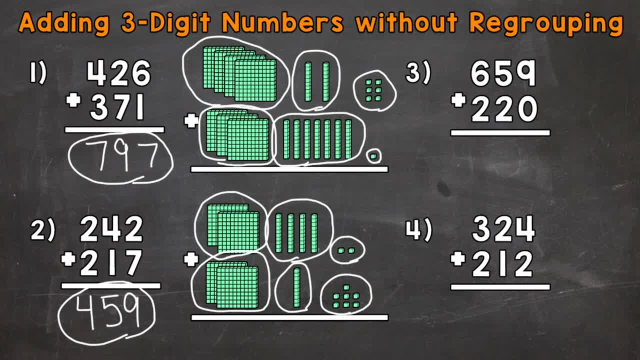 start with number 3, where we have 659 plus 220. always start with the ones. so we have 9 plus 0, that's going to give us 4- 9. then we have 5 plus 2 or 50 plus 20, that's going to give us 7 in the tens place, and then 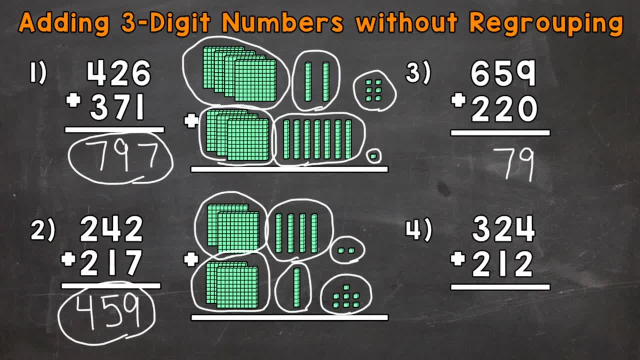 lastly in the hundreds place, 600 plus 200 or 6 plus 2 gives us an 8 in the hundreds place, our final answer is 879. and then, lastly, we have number 4: 324 plus 212. we'll start with the ones. Four plus two is six. Then we have the tens Twenty plus ten or two plus one in the tens. 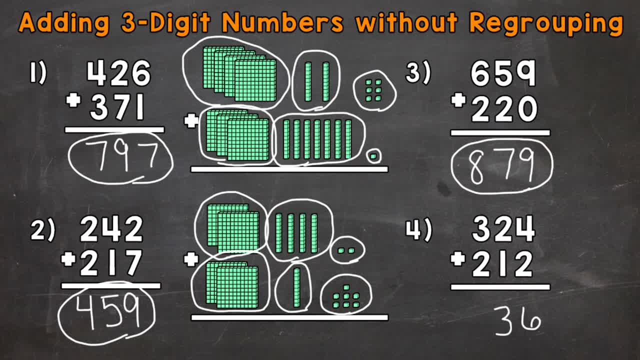 place gives us a three. in the tens place, which has a value of thirty, And then lastly, three plus two, which is actually three hundred plus two hundred. That gives us a five in the hundreds place. That five has a value of five hundred. It represents five groups of one hundred. So our 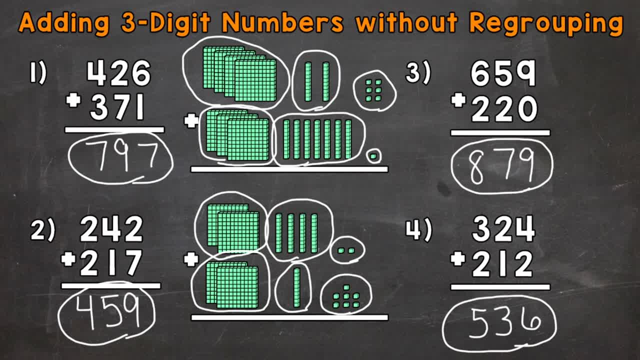 final answer is five hundred thirty-six. So there you have it. There's how you add three-digit numbers, and those problems did not involve regrouping, So I hope that helped. Thanks so much for watching, Until next time, peace.